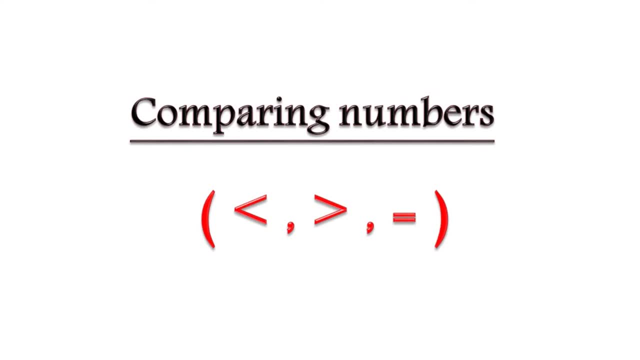 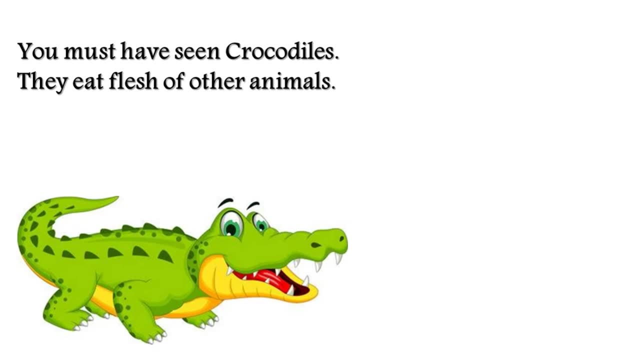 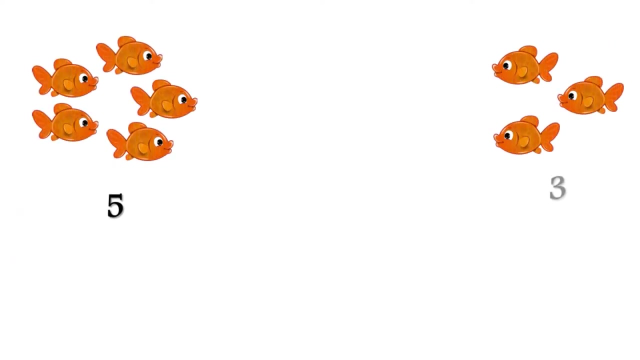 Comparing numbers. Let's see how to compare numbers using symbols. You must have seen crocodiles. They eat flesh of other animals. His wide mouth always opens towards the greater number. Here we have 5 fish on left side and 3 fish on right side. 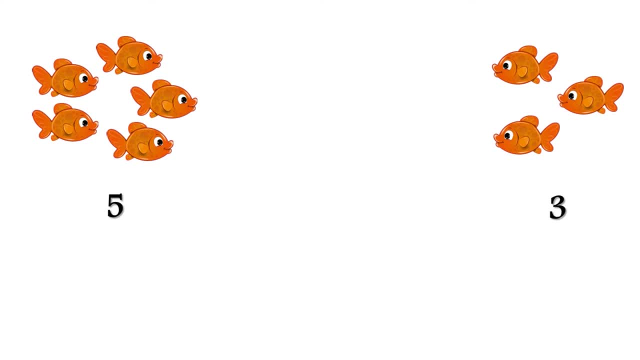 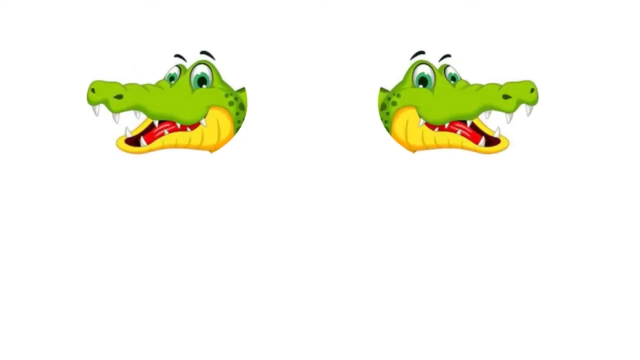 On which side crocodile will open his mouth. Yes, towards number 5.. It is written as 5 greater than 3.. Crocodile always opens his wide mouth towards the greater number and the back of his mouth will point towards small number. 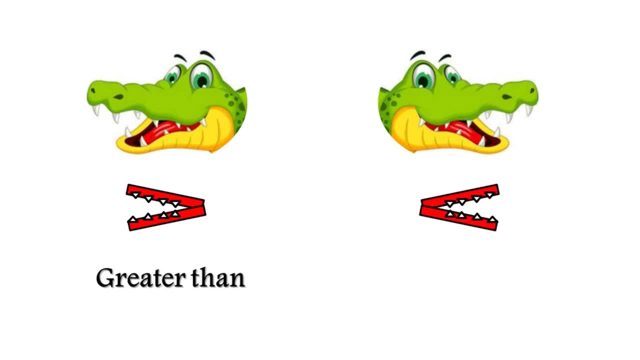 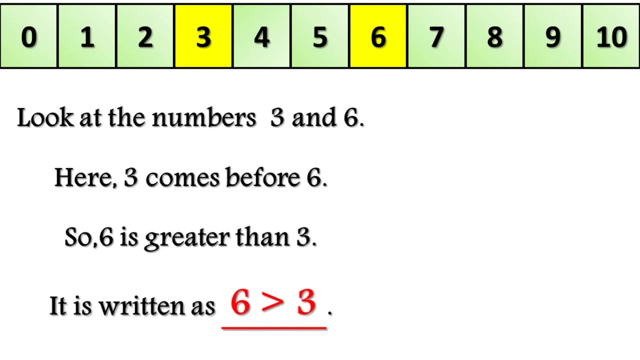 This sign is for greater than and this sign is for less than. Look at the numbers 3 and 6.. Here 3 comes before 6.. So 6 is greater than 3.. It is written as 6 greater than 3.. It is the symbol of greater than. 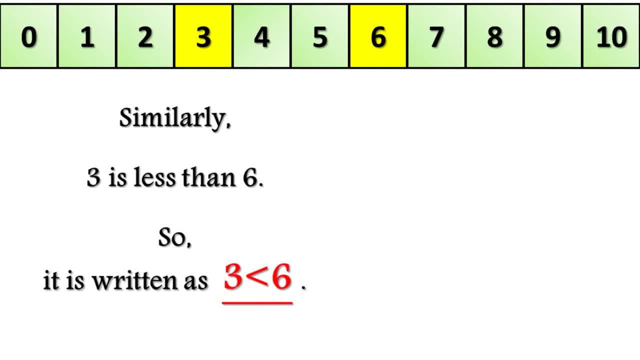 Similarly, 3 is less than 6.. So it is written as 6 greater than 3.. Similarly, 3 is less than 6.. So it is written as 6 greater than 3.. It is the symbol of greater than. 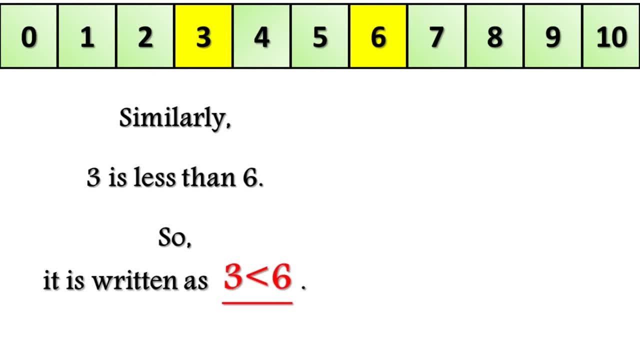 Similarly, 3 is less than 6.. So it is written as 6 greater than 3.. It is the symbol of greater than. written as 3 less than 6, it is the symbol of less than. remember this symbol if. 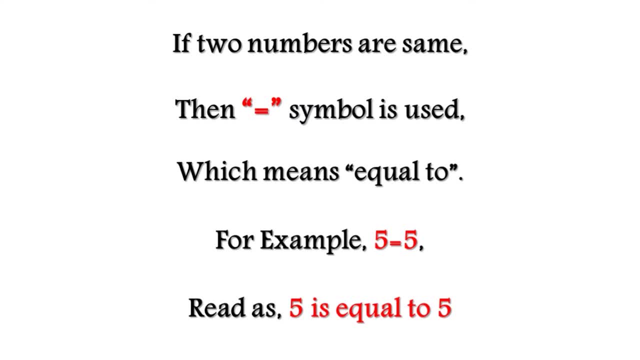 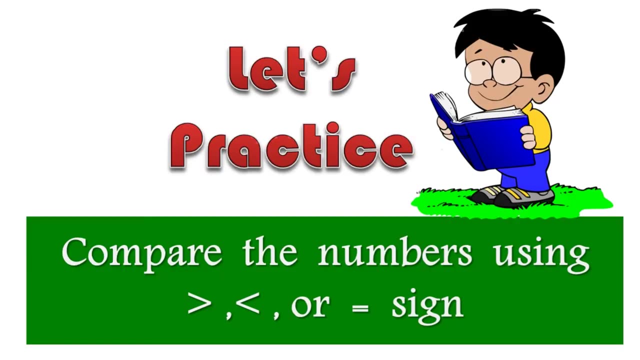 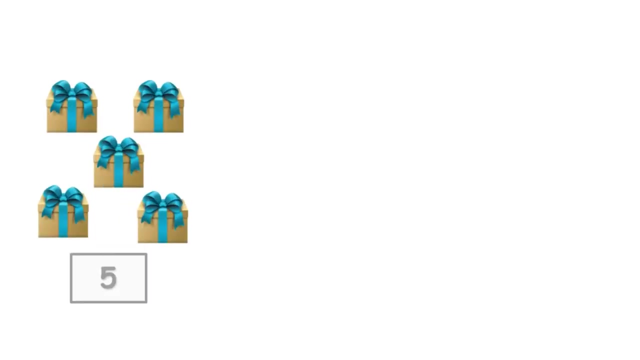 two numbers are same, then this symbol is used, which means equal to. for example, 5 is equal to 5, read as: 5, is equal to 5, let's practice here we have 5 gift. 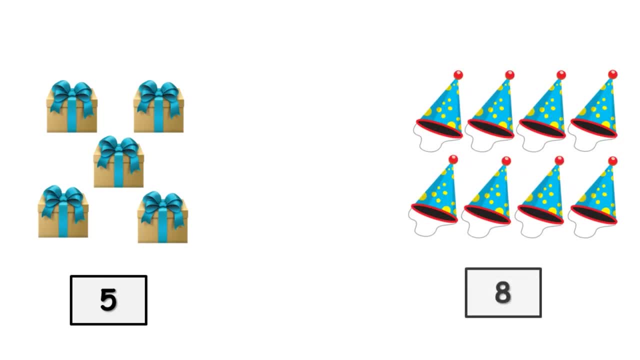 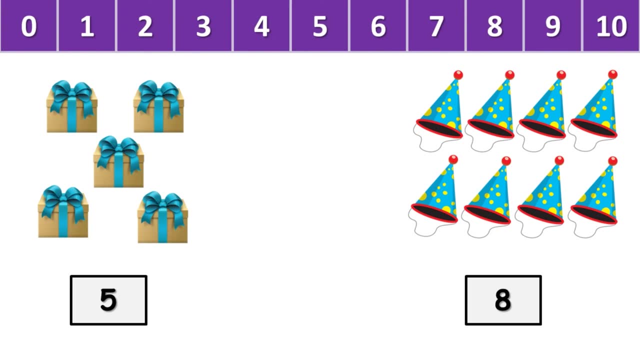 boxes on left side and 8 birthday caps on right side. and we know that a numbers strip, number 5, comes before number 8,. so where will crocodile open his mouth towards big number 8, and the? 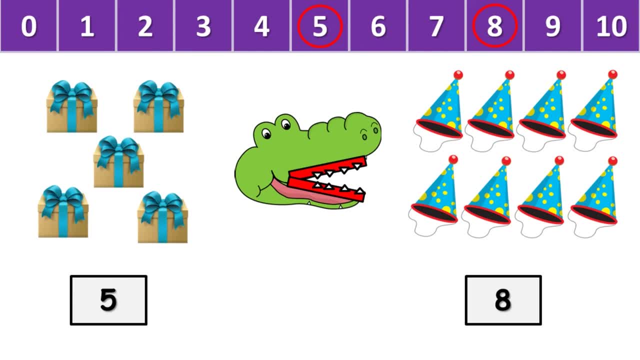 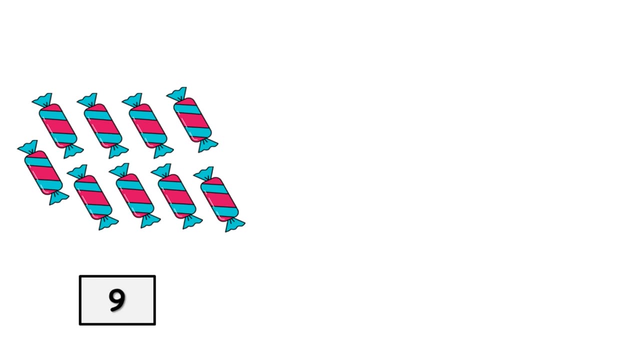 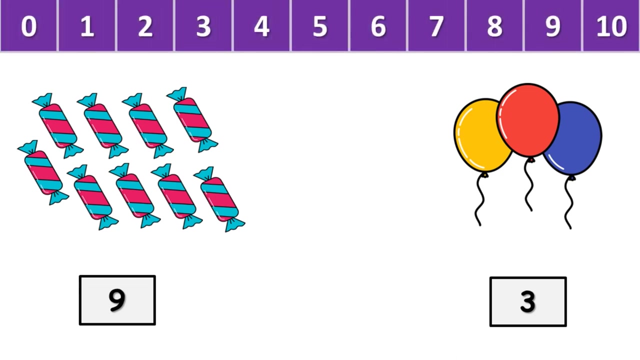 back of his mouth will point towards small number 5,. it is written as 5, is less than 8, here we have 9 candies on left side and 3 balloons on right side, and we know that a numbers strip, number 9, comes after number 3, so 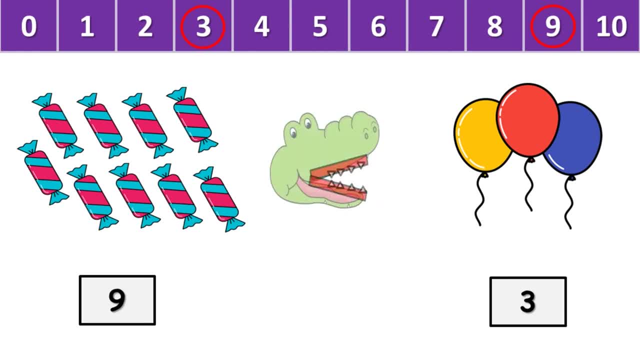 where will crocodile open his mouth? towards big number 9, and the back of his mouth will point towards small number 3,. it is written as 9, is greater than 3.. 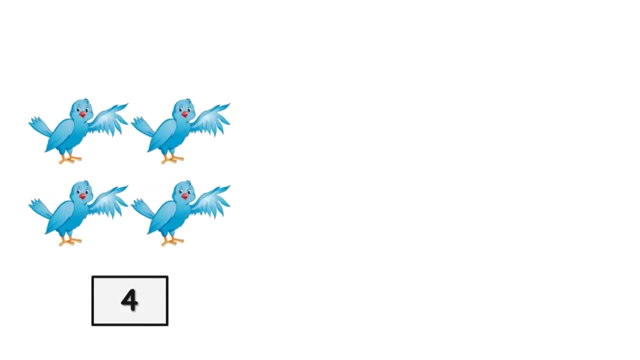 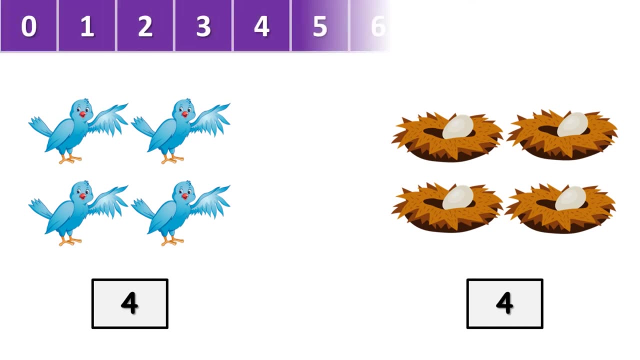 here we have 4 birds on left side and 4 nest on right side. that means 4 is equal 4, as we have the same number on both sides. so let's put the equal to sign here between: 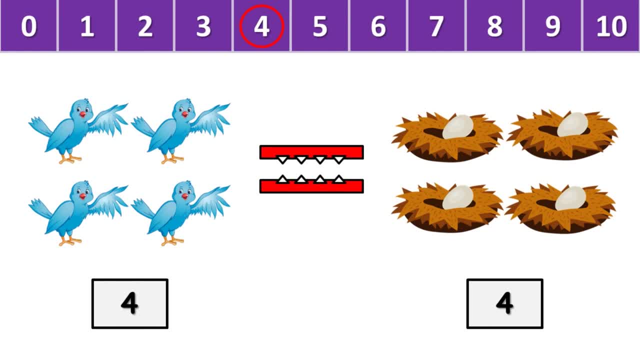 4 and 4.. it is written as 4 is equal to 4.. here we have 4 birds on left side and 4 nest on right side. that means 4 is equal. 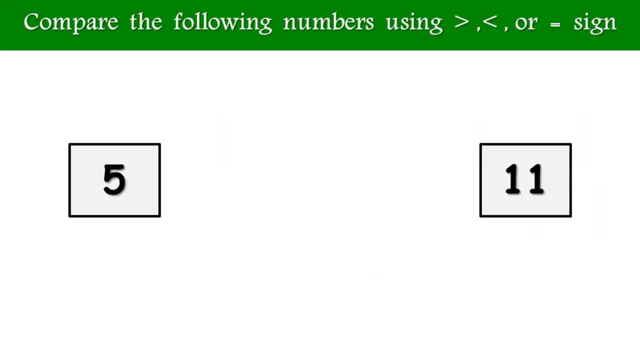 4. here we have 4 birds on left side. that means 4 is equal 5, here we have 4, can be 6, here comes 10, it is written as cat 10 and 1 it is. 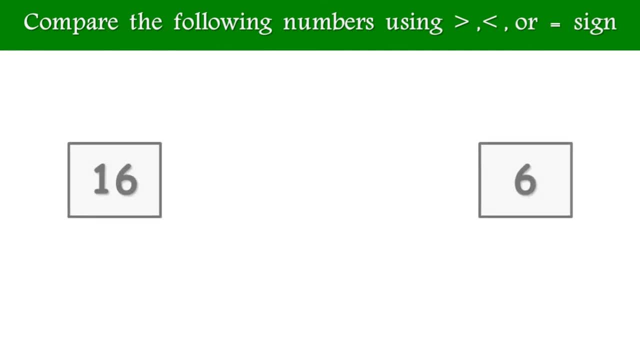 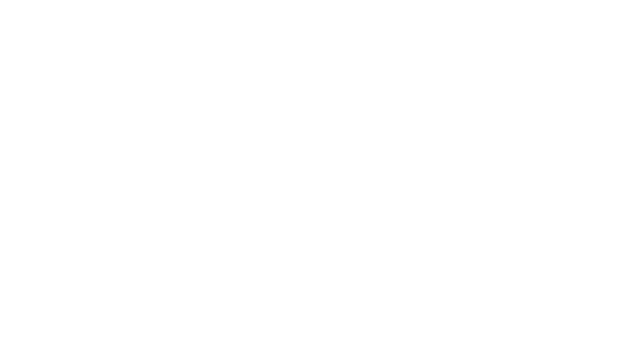 written as 4, asacia, cat 9, 1. it is written as cat 9, remained 5 birds on your other side of of the star, about 52 to remains fat 15 and 20, X we have. 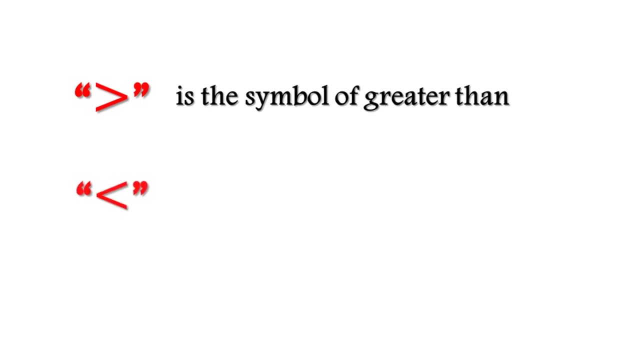 It is the symbol of greater than It is the symbol of less than. It is the symbol of equal to. If you like this video, please subscribe our channel.